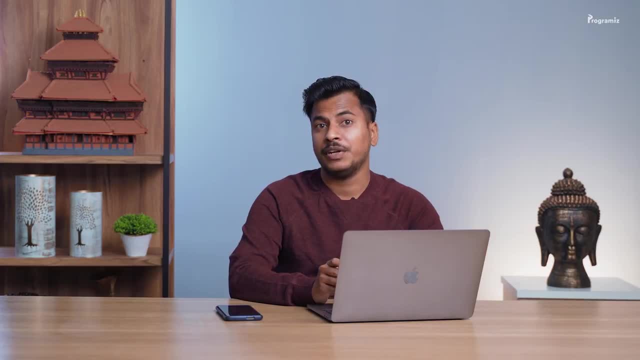 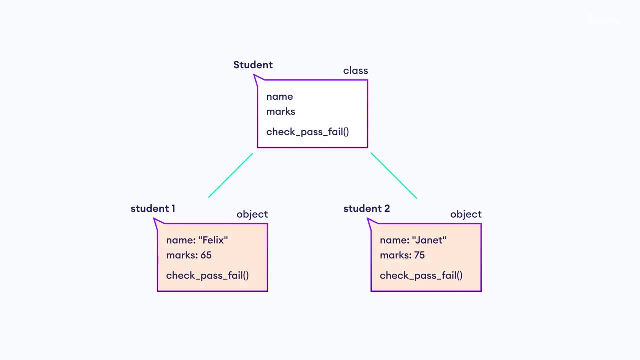 As many houses can be made from a house's blueprint, we can create many objects from a single class. So from our student class we can create as many student objects as we want. The concept of object-oriented programming is not native to Python and is available to. 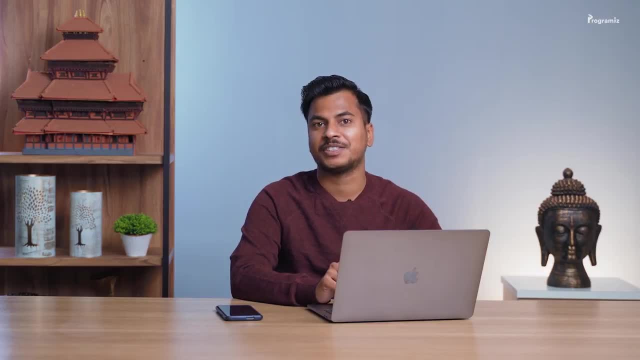 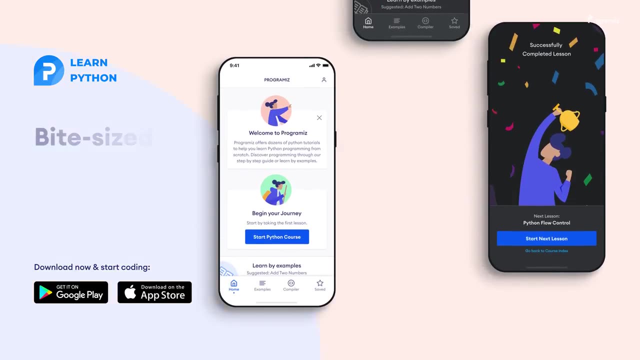 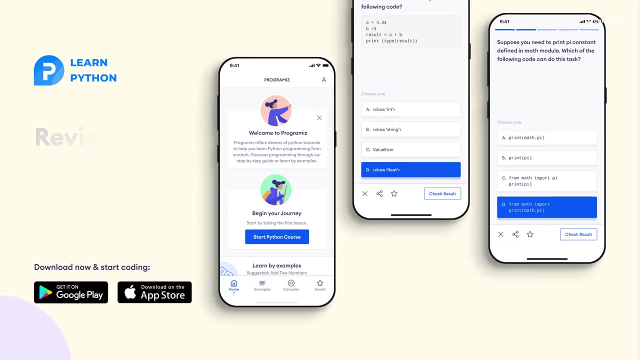 most of the programming languages. Before moving to the next section of the video, the programmers team has created an app that allows you to learn Python from your phone. The app contains bit-sized lessons that are easier to understand, a built-in interpreter so that you can run Python on your phone, quizzes and many more. 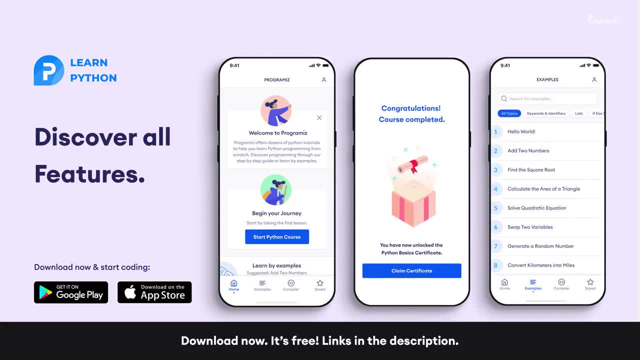 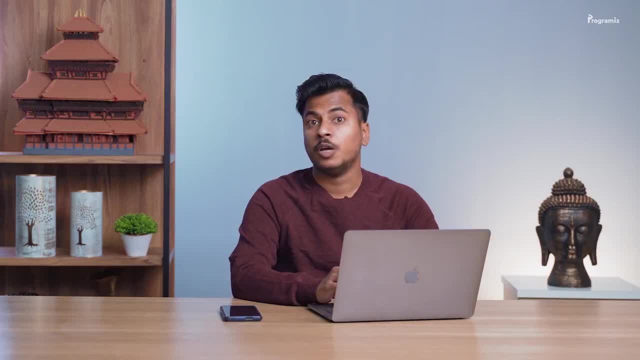 The app is available on both iOS and Android. The links are in the video description. Now that we know what objects are, let's implement them in Python. As mentioned before, we need to define a class before we can create objects. Let's do that first. 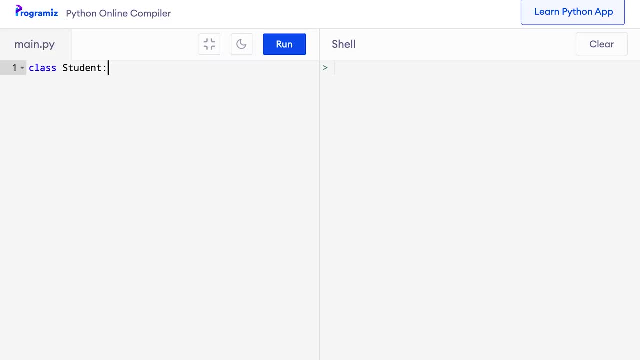 And here I'll say class student and then I'll just use pass. Here I have defined a class named student. At the moment, our class doesn't have any attributes and methods. Since classes cannot be empty, I have added a pass statement. 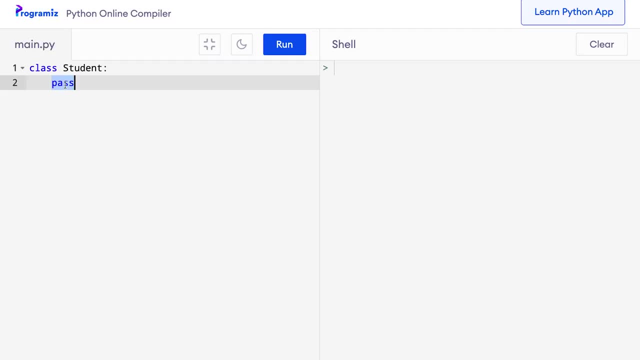 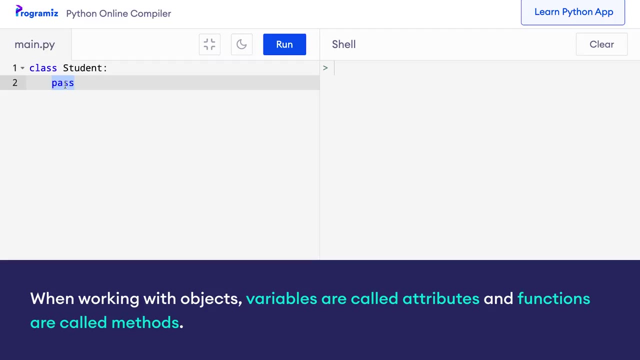 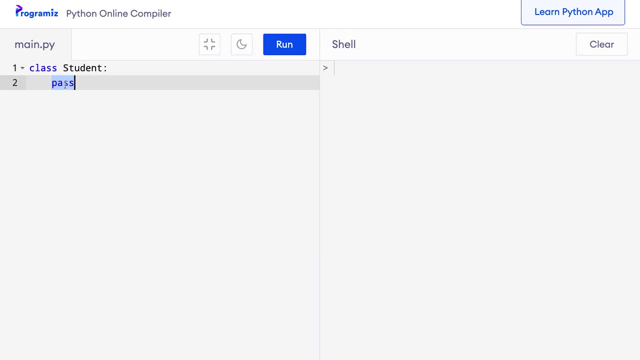 So that I can run the code without any errors. By the way, when working with objects, variables are called attributes and functions are called methods. From now on, we will be using these terms when working with objects. Now that we have defined a class, we can create as many objects as we want from it. 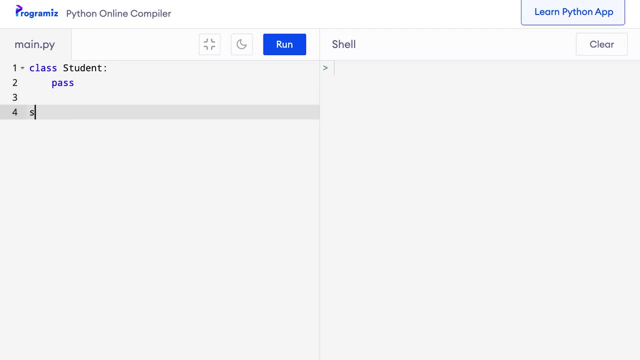 Let me create two objects of the class. I'll say student1 equals student, and then I'll say student1 equals student, and then I'll say student1 equals student. Here I'll say student1 equals student, and then I'll say student2 equals student. 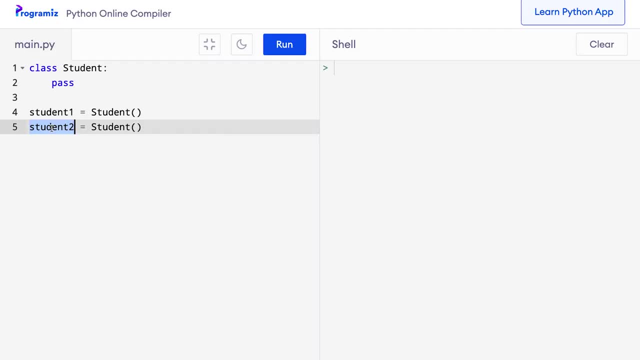 Here, student1 and student2 are both objects of the student class. Now we can start adding different attributes to these object instances. First let me remove the student2, and here I'll say: student1.name equals harry …. … harry to the name attribute of the student, one object. let me add another attribute to our object. 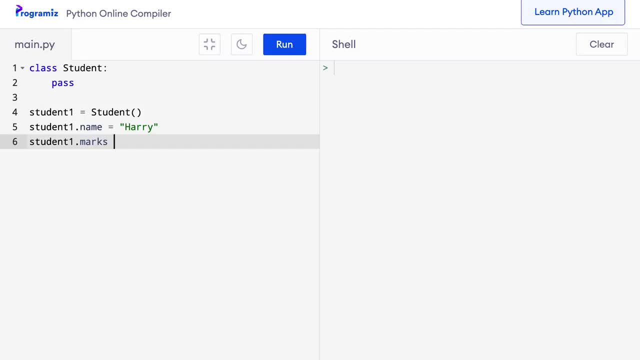 so here i'll say student 1 dot marks equals 85 and i'll print these attributes. i'll say print student one dot name and print student one dot marks. now when i press run i get harry and edify back. we have successfully added two attributes to a student one object. however, this is not the. 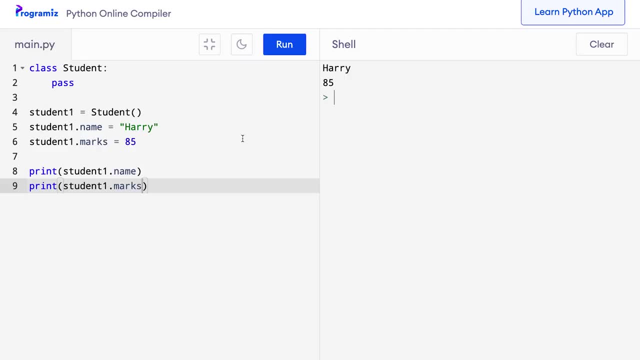 proper way to add attributes to objects. usually, what we want to do is we want to put attributes inside our class so that all the objects created from the class will be added to our class class have these attributes by default. similarly, we also put all methods inside our class so that 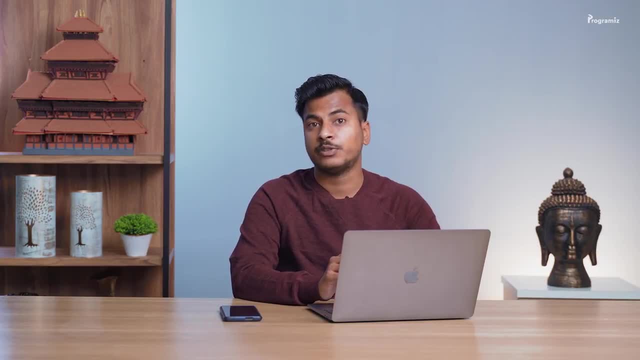 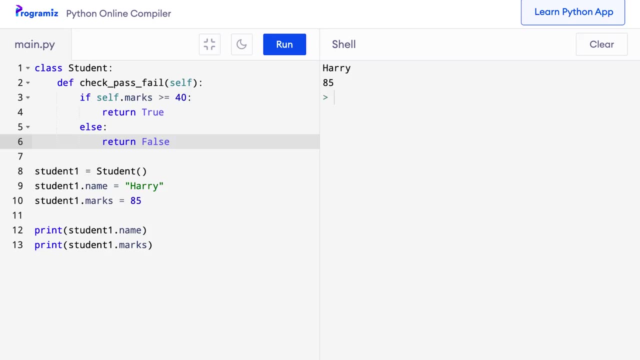 every object of the class can access them. let's first see how we can add methods inside a class. then we will look into the proper way to create attributes here. i have defined the check pass fail method inside the class. now any object created from this class will have access to the. 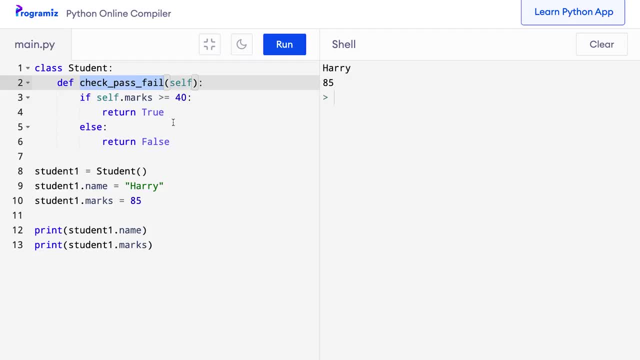 check pass fail method. if you have noticed, we have used self as an argument here and self dot marks inside the method. we will talk about that in a moment. let's first access this method using the student one object. so at the end here i'll say: did underscore pass equals? 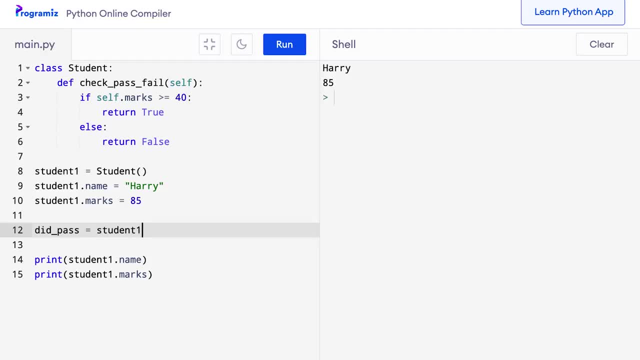 student one dot check underscore pass, underscore fail you. and then i'll say i'll remove these two lines and i'll say print did underscore pass. now, when i press run then as expected it prints true because the student one has enough marks to pass. let's see from the very beginning what's going on here. we have created a class and we have defined 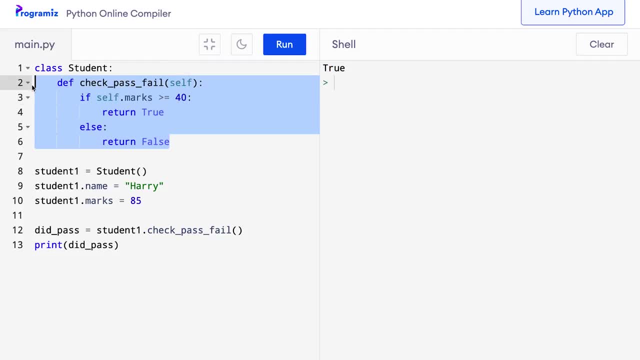 a check pass fail method inside it. then we created an object from this class and added two attributes- name and marks- to it. finally, we call the check pass fail method using the student one object. we have called this method without passing any arguments. however, the method definition has an argument called self. now you must be thinking: shouldn't this give us an error? 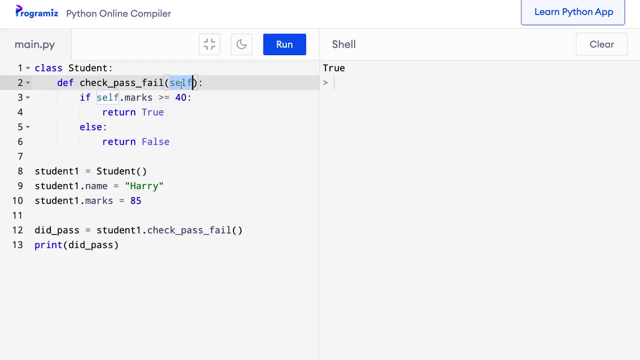 well, whenever we define methods for a class, we need to use self as the first argument. this self represents the object calling it. in our example, self refers to the student- one object, and self dot marks refers to the marks attribute of the student one object. so the object is passed as the first. 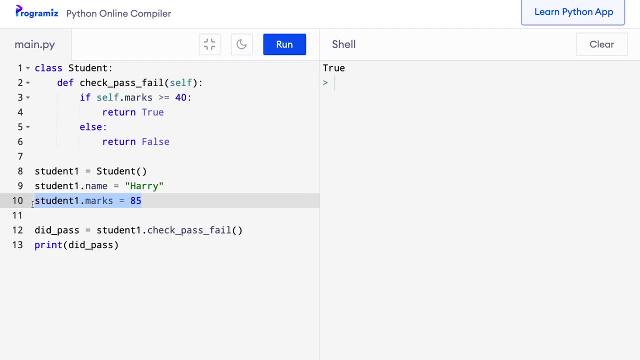 argument automatically. if we create another object, let's say student two, and call this method, then self represents the student two object and self dot marks represents the marks attribute of the student two object. let's try it out: student two equals student student two dot name equals janet student. two dot marks equals 30. 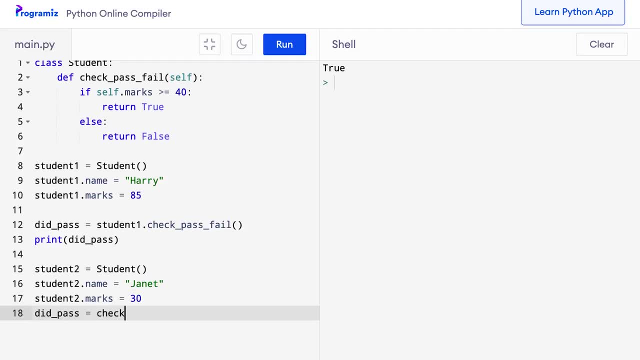 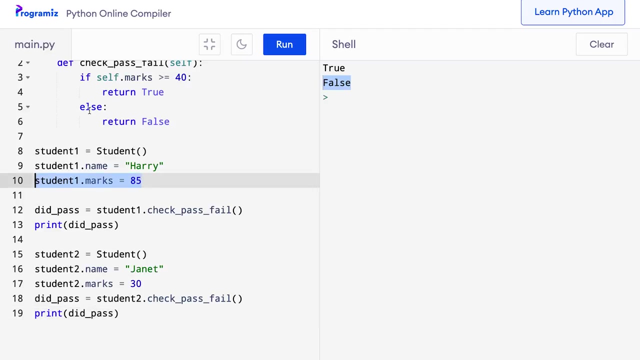 did: underscore pass equals check pass fail. oops, student two dot check pass fail. and let me print underscore pass now. when i press run, then i get true first and i get false here. marks of student one is 85, so in this method self dot marks is 85, which is greater than 40. that's why true is returned. 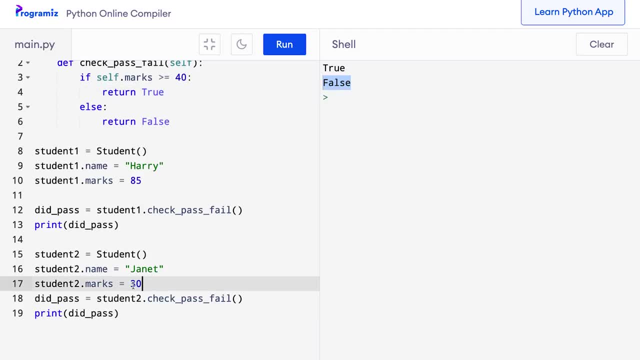 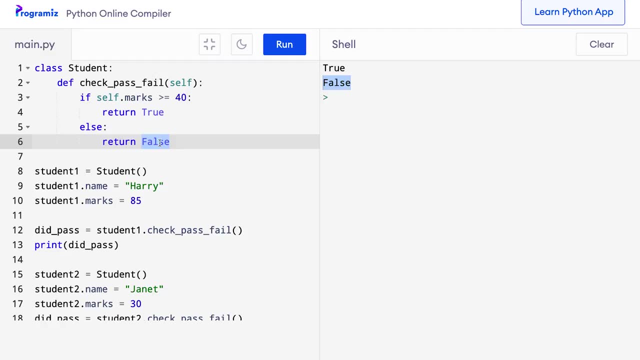 similarly for student two. student dot two dot marks is 30, so self dot marks greater than equals to 40 is false. that's why we get false. by the way, student two dot marks equals 40. that's why we get false. by the way, we can use any name instead of self here. it's just an identifier, like variable names. 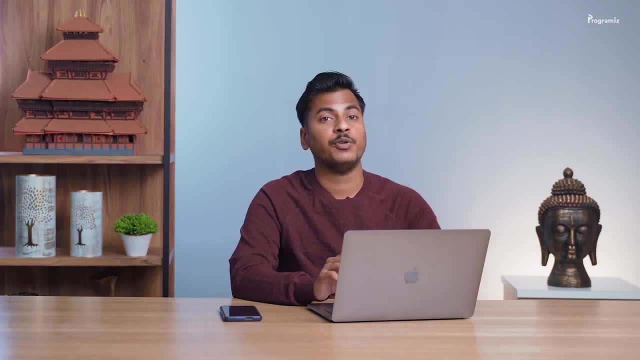 using self is a convention and for consistency, we will also keep using self. if you're finding this video useful, a sub to the channel would be awesome. as i have previously mentioned, adding attributes to the object manually after defining it is not a good practice. instead, python offers. 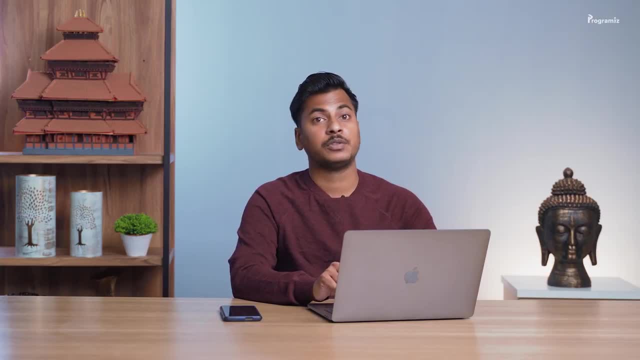 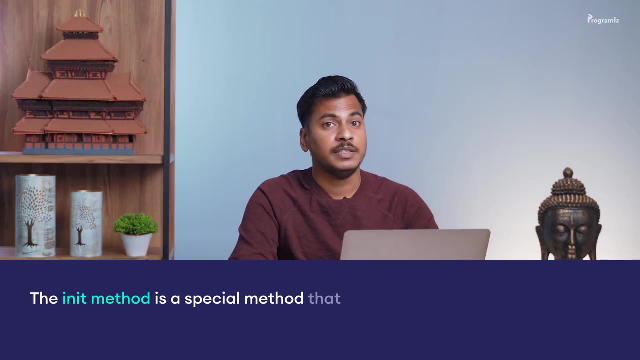 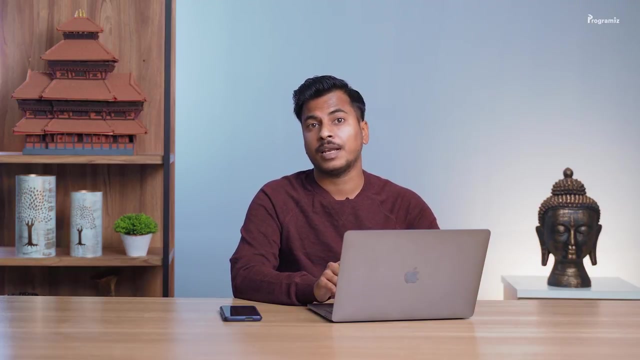 a much more elegant and compact way of defining attributes while instantiating the object. For that we use the init method. The init method is a special method that automatically gets called every time objects are created. If you're coming from other programming languages, like C++ or Java, the Python init method closely resembles constructors. 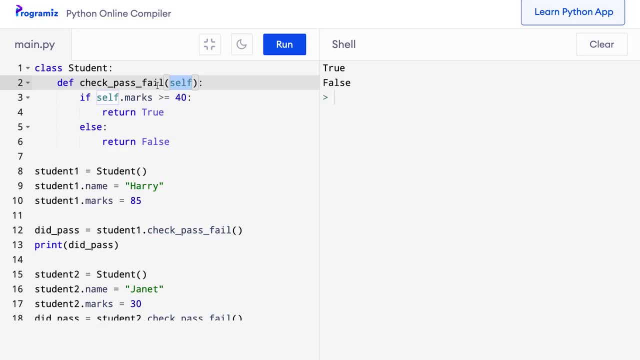 So let's see how we can use the init method in our code, And I'll remove the student2 code And I'll also remove the code that adds the attributes of name and marks to the student1 object. Then I'll say: def. underscore, underscore init. underscore underscore self name marks. 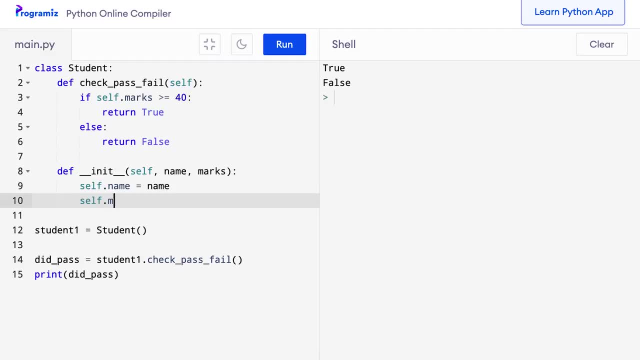 That's: a self dot name equals name, self dot marks equals marks. And here I'll see Harry and 85. Now let me also remove this did pass And I'll say: print student one dot name and print student one dot marks. Let's see what's happening here. When we create an 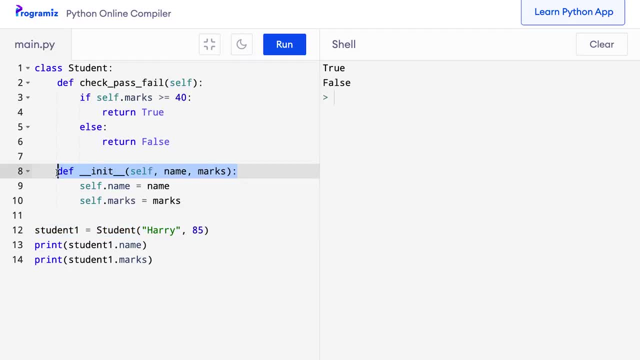 object. This init method is called automatically with the values Harry and 85 passed to name and marks automatically. Remember, the first parameter self represents the object calling it, while the second and third parameter take the two arguments which we use during object creation. Now for the student one. 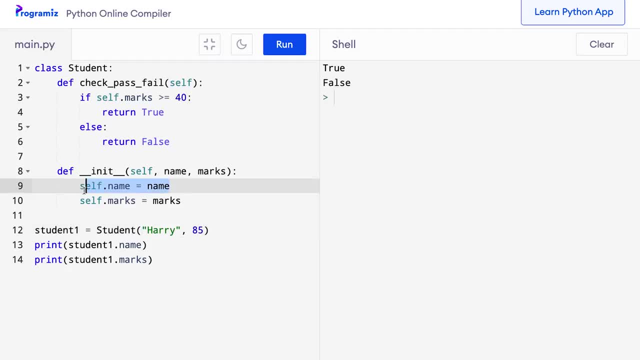 object. the name attribute will be Harry because of the statement self dot name equals name and marks will be 85 because of the statement self dot marks equals marks. When I run this code, get Harry and 85.. Let's create another object. First I'll add another student, student two. 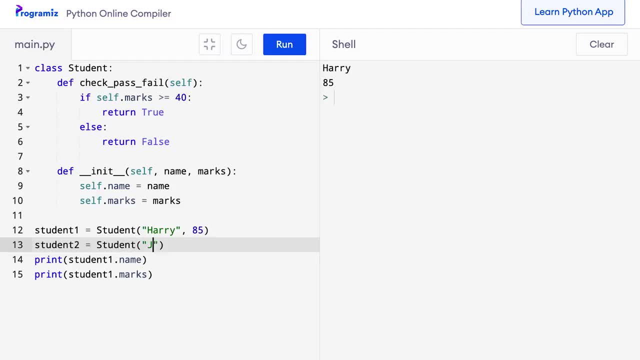 equals student Janet, 30. Let me print those. So I'll say: print student to dot name and print student to dot marks. Now when I press run then I get Harry 85, Janet and 30. Now let me check if student one and student two passed or failed the exams. We already have the 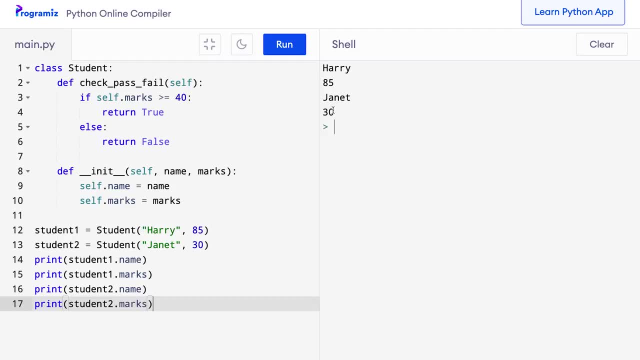 check pass fail method defined for this purpose. We just need to call it. But first I'll remove the code to print the attributes And then I'll say did underscore pass equals student one dot check pass fail. Let me print did underscore pass And again I'll modify did pass so that I know. 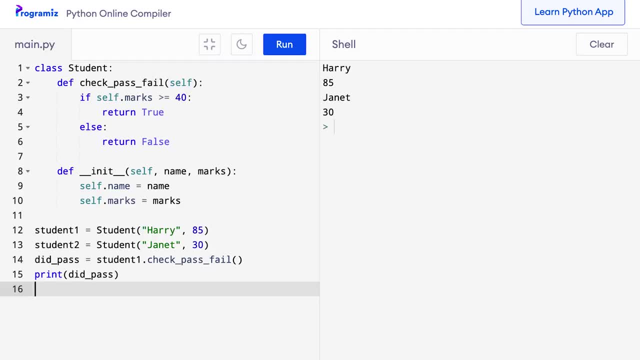 the value or the pass fail. status of state: student two. So I'll say: did underscore pass equals student two. dot check Pass fail Print: did underscore pass? You must have guessed the output by now, But let me run the code and verify anyways. So I'll press run. 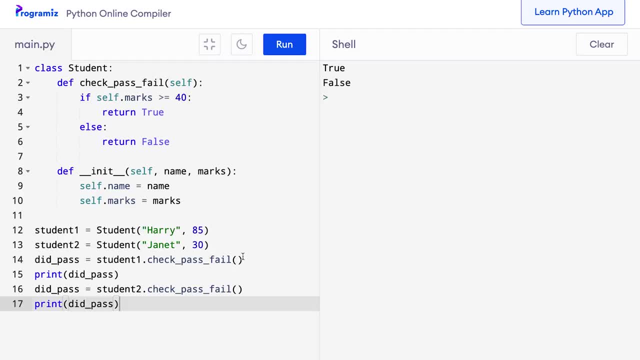 And, as expected, true and false are returned Because in this line did underscore pass will be true since the first student, Harry, has enough marks to pass the exam. Similarly, here did pass will be false because student two does not have enough marks to pass. 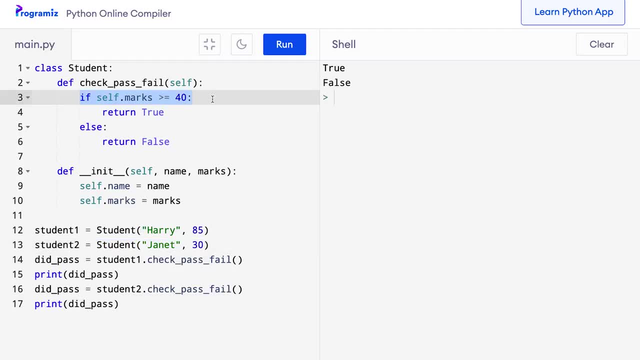 the exam. Let's see how this program works from the very beginning again. We have created a class with two methods: and init method that initializes the attributes of name and marks, And a check pass fail method that returns true if the marks is greater than 40, greater. 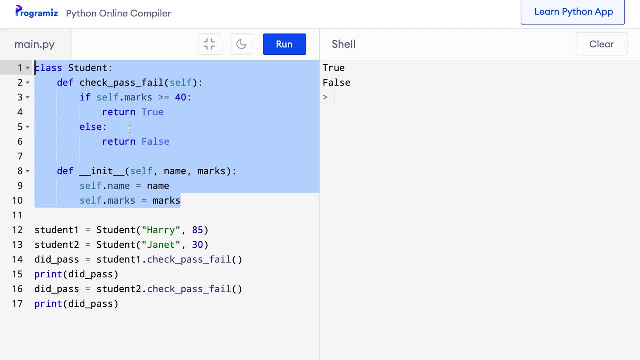 than equals 40 and false if it's not greater than equals 40. We then create a student one in this line with the parameters Harry and 85. When this object is created, the init method is called and name and marks attributes of this student one object are now Harry and 85. Then we check if 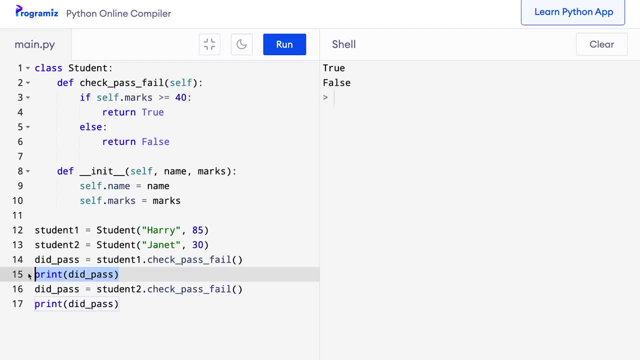 the student one passed the exam and printed the result. We had also created another object, student two, by passing Janet and 30. So the name and marks of the student two object are Janet and 30. And then we calculated if the student had passed or not using the check pass fail method. 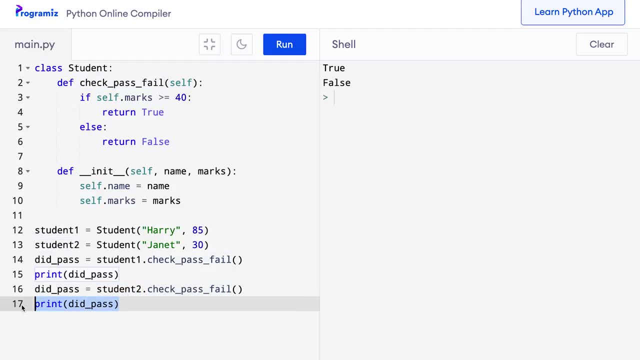 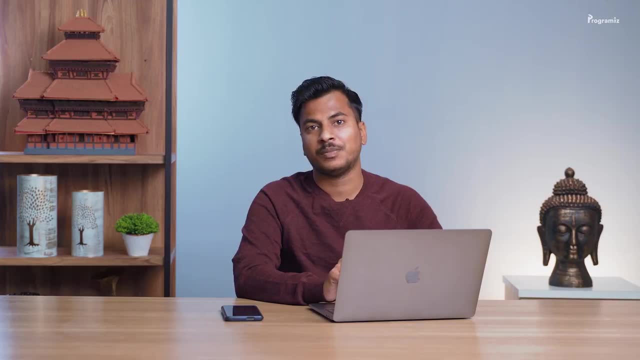 of the student two object and we printed the result. I hope you have some idea of how classes and objects work by now. Let's try one more example for extra clarity. I hope you have some idea of how classes and objects work by now. Let's try one more example for extra clarity. 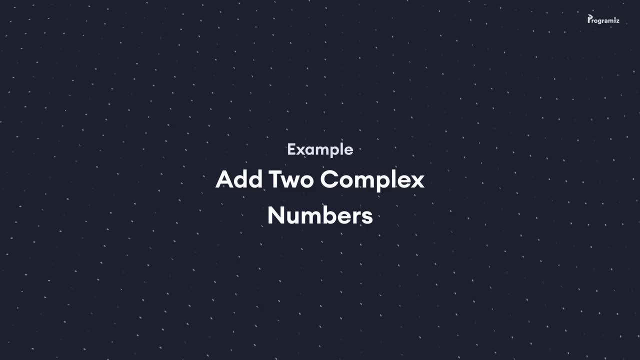 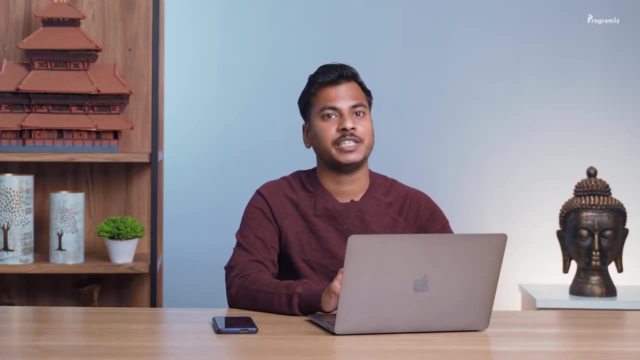 In this example we will add two complex numbers manually. Python already handles this by default, but we will create our own complex class to better understand the concepts of object-oriented programming. If you do not know, a complex number has real and imaginary parts. 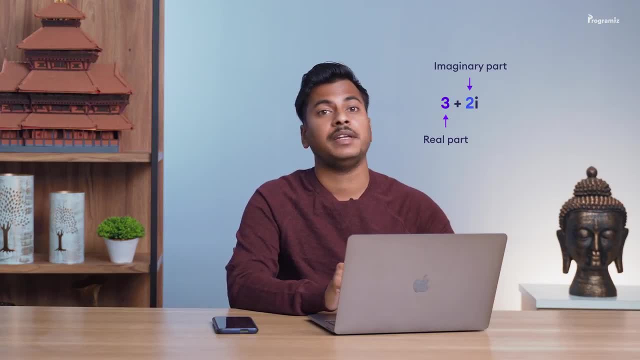 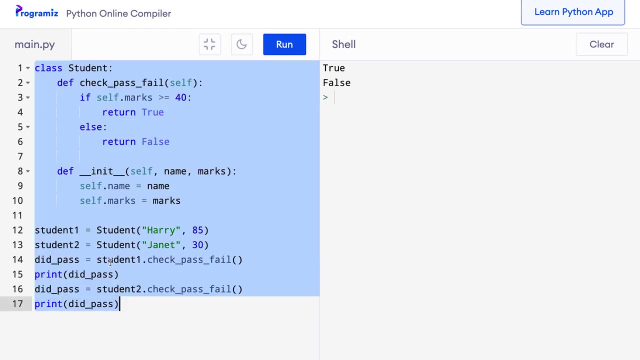 When we add two complex numbers, we need to add the real and imaginary parts separately. Let's first create a class that represents complex numbers. I'll remove this old code and I'll type class complex and here I'll define an init function. so i'll say def- init. 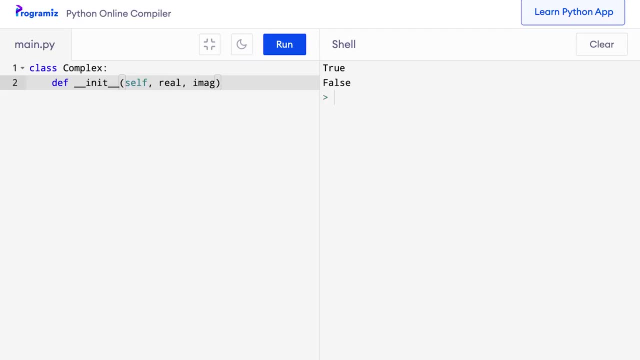 self real image. and inside this i'll say: selfreal equals real and selfimaginary equals image. and now let me create two objects: n1 equals complex five, five, six, five, six, five, six and n2 equals complex minus four and two. at this point we have created two complex numbers. 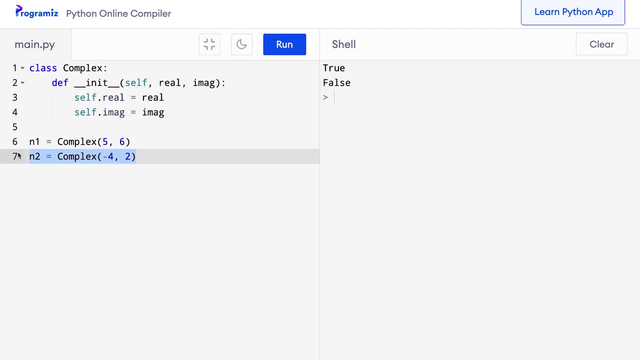 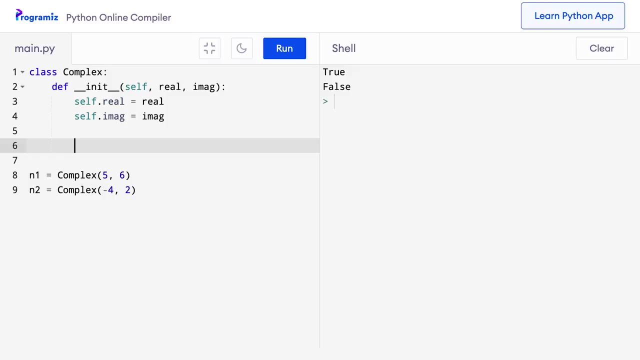 n1 and n2 and initialize the real and imaginary parts. now we'll create a method to add these complex numbers. so inside our class i'll add the code, i'll say def- add self number and here i'll say real equals self dot real plus number dot real. and i'll say image equals self, dot image plus. 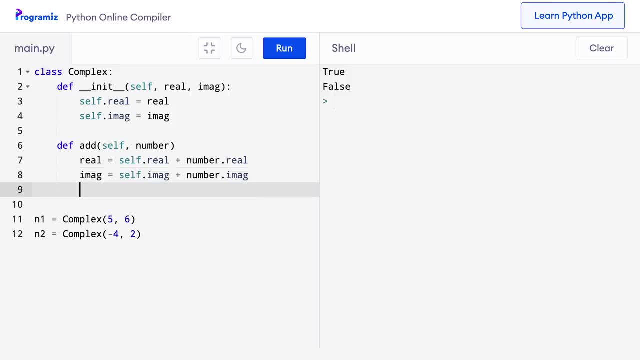 number, dot image. then i'll say: result equals complex real image and i'll return this result object. now let me call the add method. so here i'll say: result equals n1 dot add n2. here we have called the add method on the n1 object and 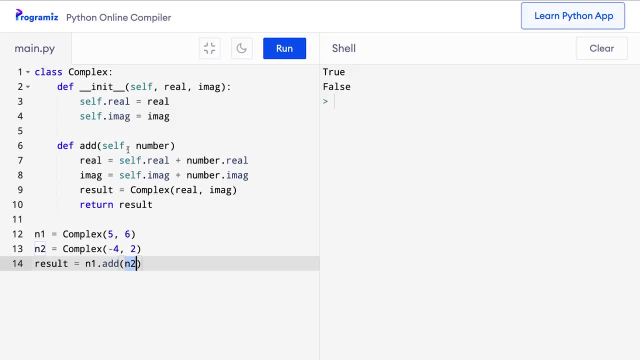 pass the n2 object to it. so inside the add method self will be n1 and number will be n2. then the real and imaginary parts of these numbers are added separately. so real equals self dot. real plus number dot. real means n1 dot. real plus n2 dot real. similarly, image equals self dot. image dot plus number dot image. 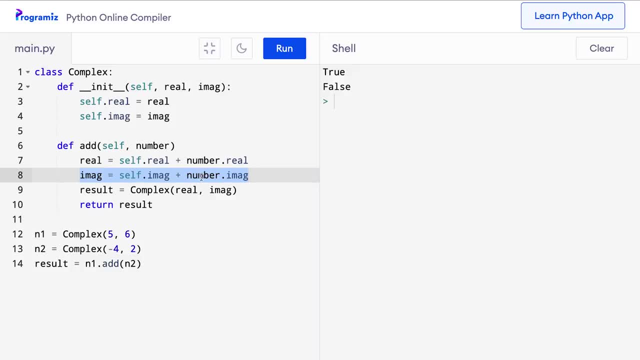 means n1, because n1 is self n1 dot image and number is n2, so n2 dot image. we have then created another object of the complex class using the result values and then returned it in the next line. now let's print the attributes of the result object. i'll say: print real equals. 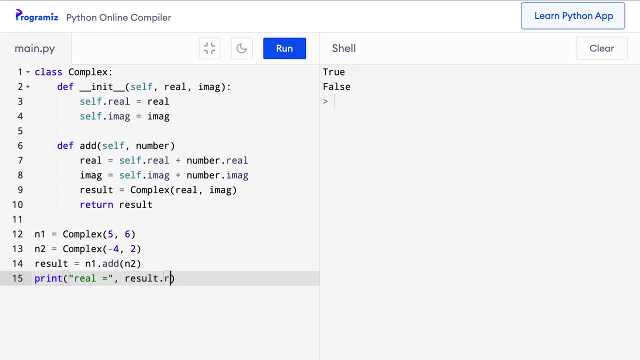 result: dot: real and print image equals result: dot: image. now when i press run, this seems to be problem. i forgot the colon. now when i press run, then i get real equals 1, image equals 8.. let's verify. so 5 minus 4 is 1 and 6 plus 2 is 8. so the answer is correct. 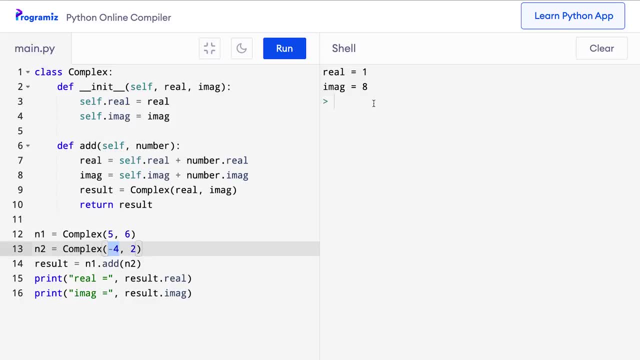 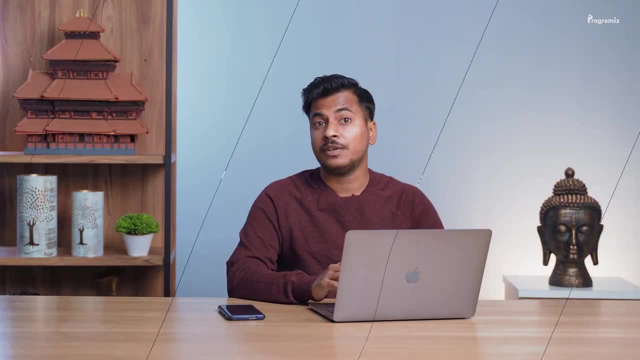 as you can see, the real and imaginary parts have been added separately, as expected. why? object oriented programming? as we have seen from our examples creating objects, allows us to organize related data and functionalities together. this helps us to write structured and flexible code now, instead of thinking in terms of individual data and functions. 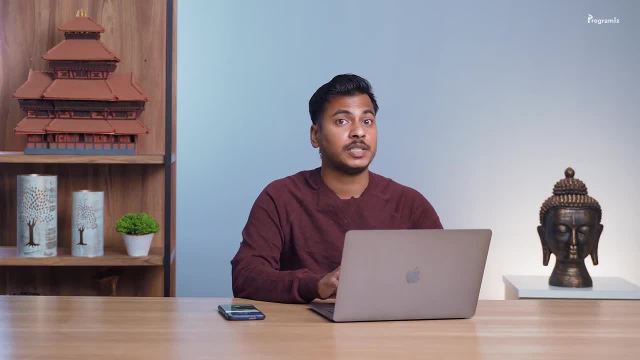 we start thinking in terms of objects and how one objects interacts with the other. this helps us to divide a complex problem into smaller sub-problems. also, using an object-oriented style of programming makes our code reusable, because we can define multiple objects with similar attributes and functionalities from a 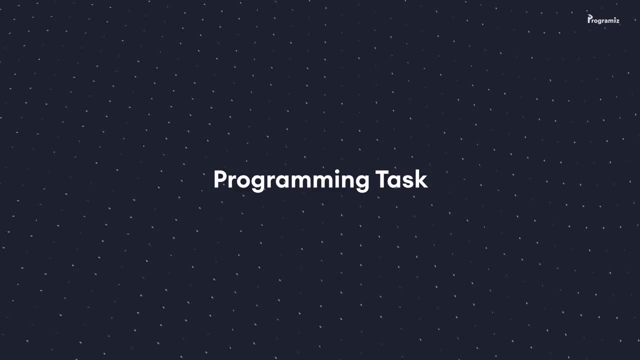 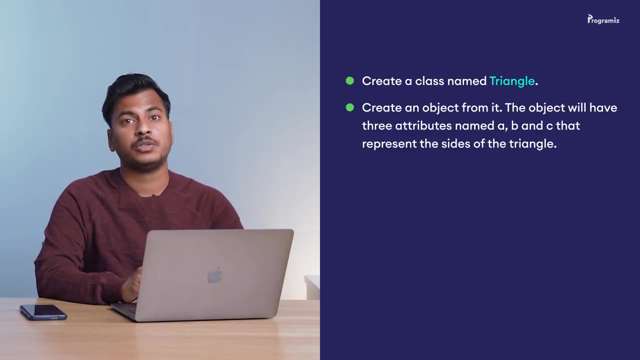 single class. before we end this video, here's a task for you: create a class named triangle. create an object from it. the object will have three attributes, named a, b and c, that represent the sides of the triangle. below we have three attributes named a, b and c that represent the sides of the triangle. 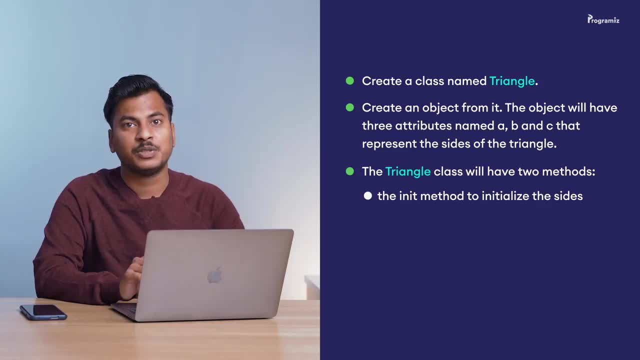 The triangle class will have two methods: the init method to initialize the sides and a method to calculate the perimeter of the triangle from its sides. The perimeter of the triangle should be printed from outside the class. Here's the bare bones code for the program. 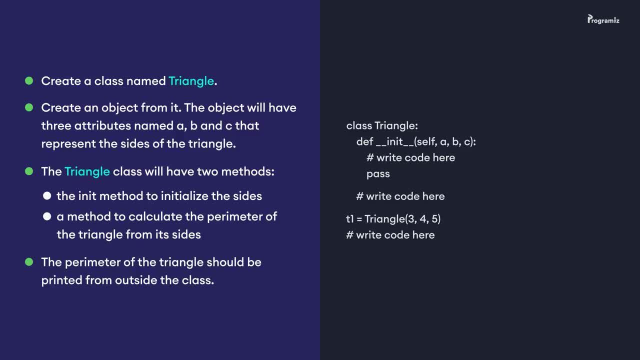 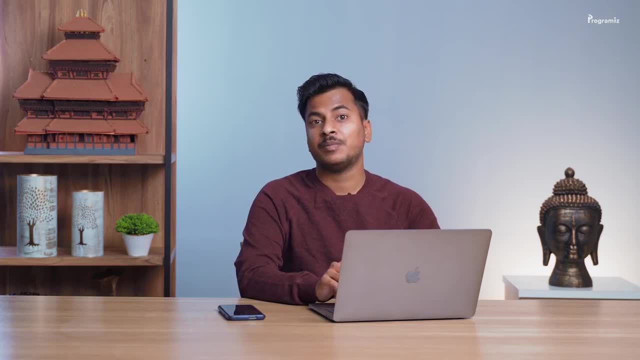 You'll find the complete answer to this question, along with source code of all the programs in this video in our GitHub repository. The link will be in the description below And, if you like this video, hit the like button and subscribe to the channel and I'll see you in the next one. Happy programming.